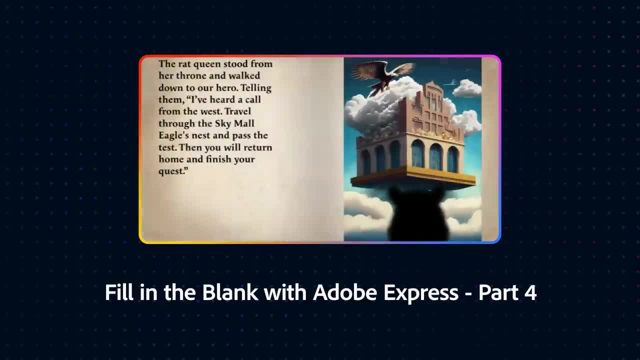 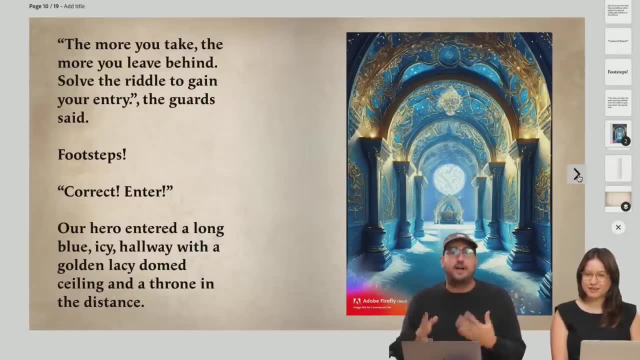 Today we are going to be continuing our story. I have written part of the story and you get to fill in the blank. We will be filling it together and creating some graphics and some generations using Firefly. We have this in Illustrator. This is where we have been working in the past. We are 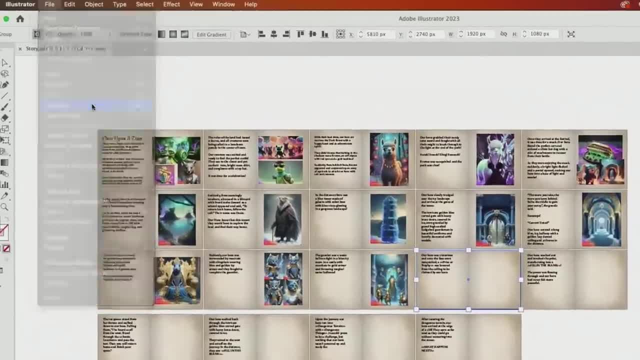 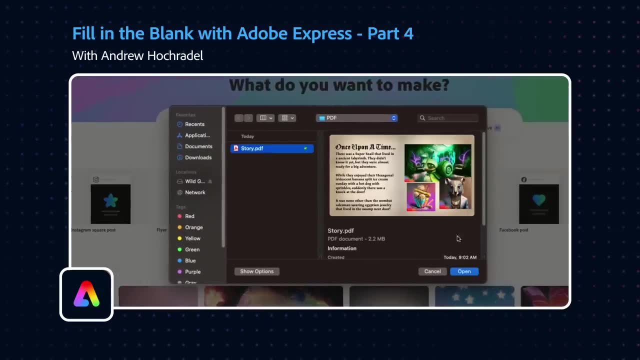 going to take this into Express today, So we're going to file and then go to save as and we're just going to export this as a PDF. We're going to go here and we are just going to click on start from your content and we're going to upload this PDF. So we have our story here. You can see the. 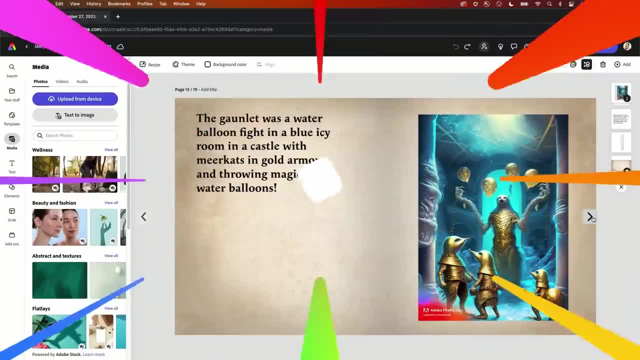 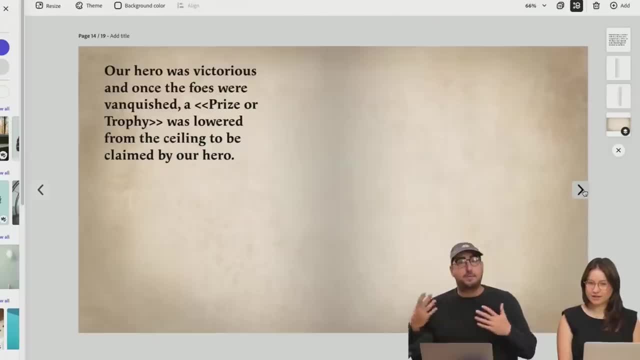 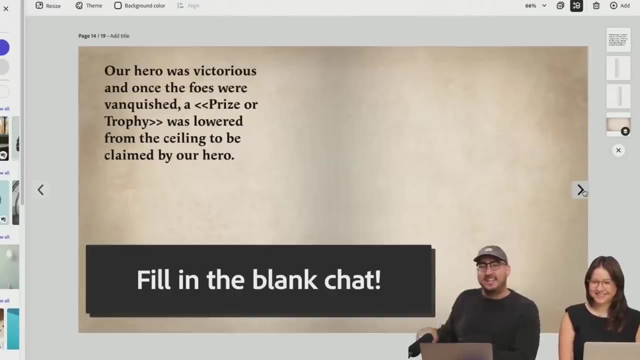 PDF actually brought in all of our different pages. Here's where we leave off our hero and where we start our story. Our hero was victorious and once the foes were vanquished, a prize or trophy was lowered for the ceiling. It's time for you chat to fill in the blank. What is the 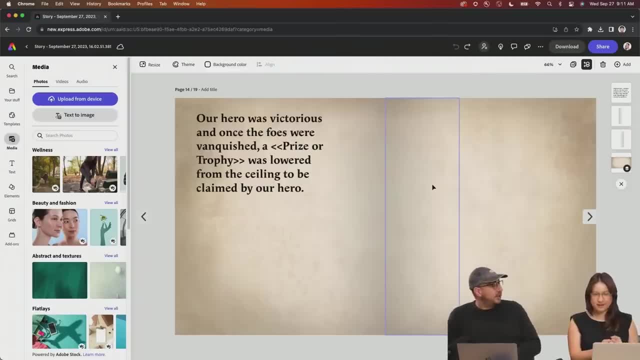 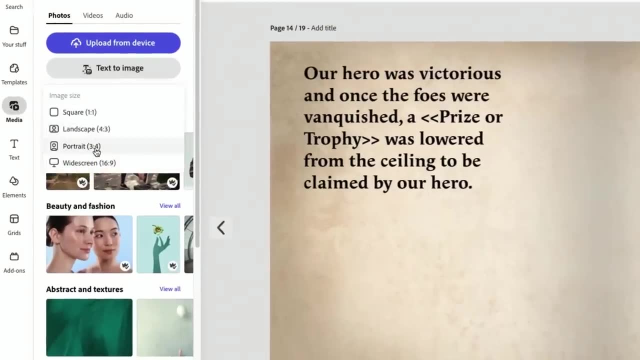 prize or trophy- Oh, it's chips Like a nacho, It's like a super nacho. prize: trophy goblet. Let's do that. So we're going to click on media here and do text to image, And I do want to do. 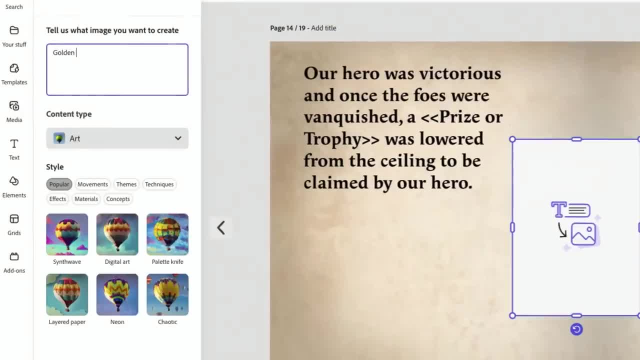 a portrait Which is three by four, Maybe a golden goblet filled with cheese and chips. Let's do photo here to try to make it photo realistic. And then I also like to add in photo realistic: Between your different pieces you want to put commas. So here we go, Let's generate. 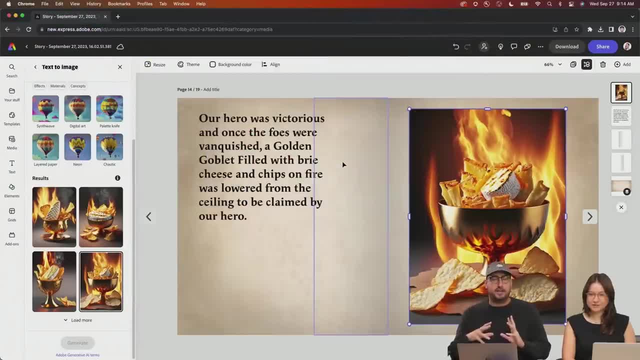 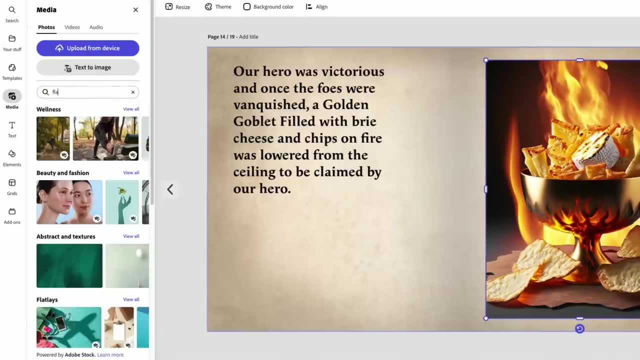 the nacho goblet. We are going to use Adobe Express to put some video on top of this. We're going to go over to media and I'm going to type in flames on black background And I want to do video And we are just going to upload this. So we're going to go over to media and I'm 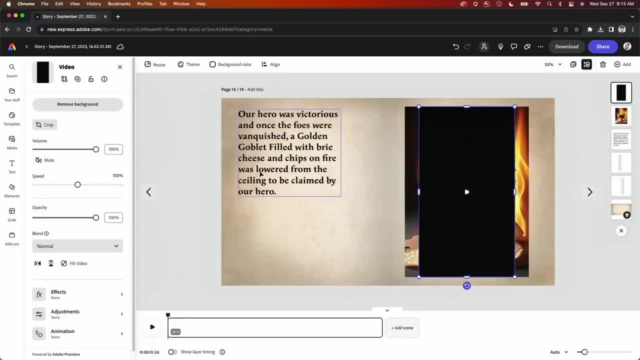 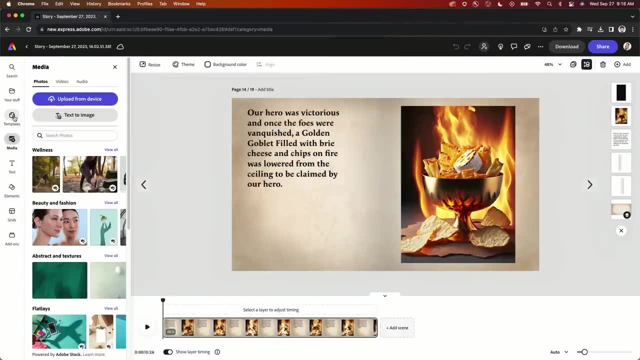 going to type in flames on black background And I want to do video And we are just going to overlay this over our image And then we're going to change the blending mode to screen. Yes, We are going to add some music to this clip. Let's go to media and I'm going to do audio and 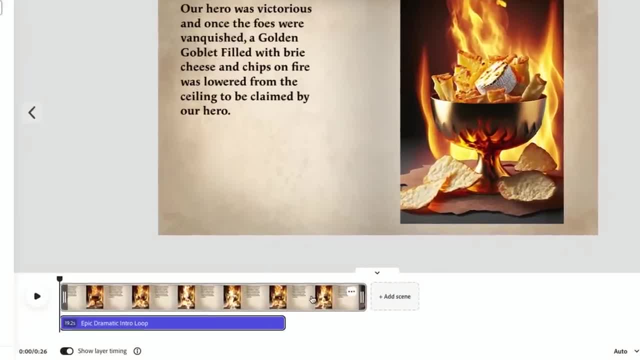 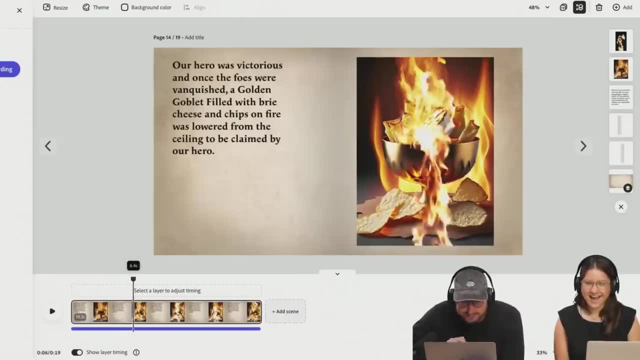 we're just going to type in epic, So I'm going to click that and it will pull it all the way in. Here is where I'm going to record my voiceover. I'm going to click on voiceover right here. Golden goblet filled with brie cheese and chips on fire was lowered from the ceiling. 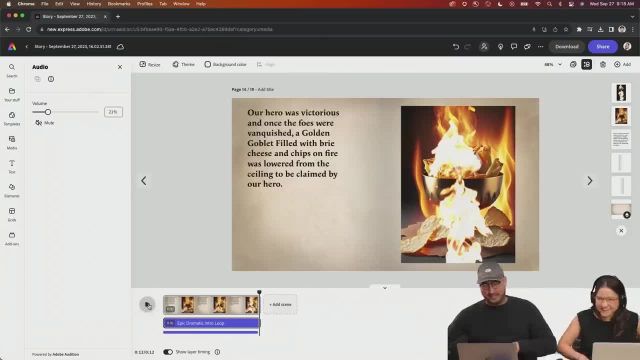 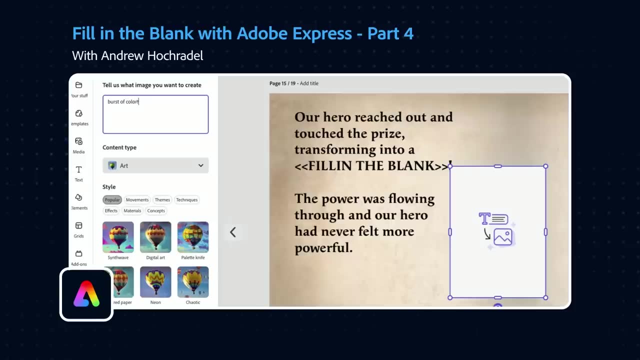 to be claimed from our hero. So fun. This is my favorite stream ever now. Okay, Moving on to our next page. So let's do the background first. burst of colorful lightning- Oh, these are great. I'm actually going to keep a couple of these. 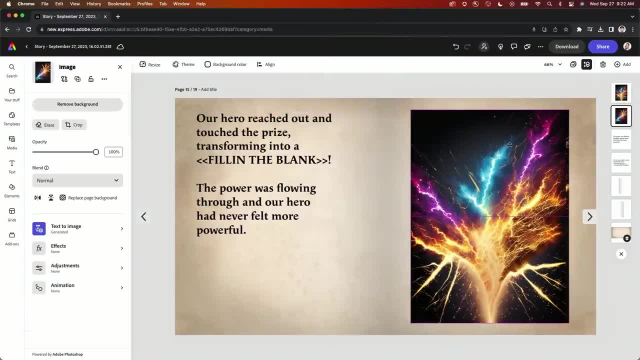 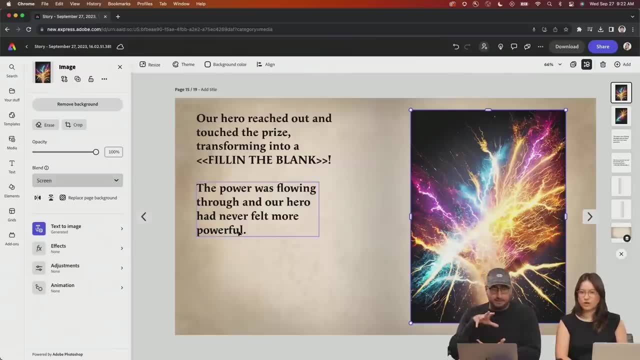 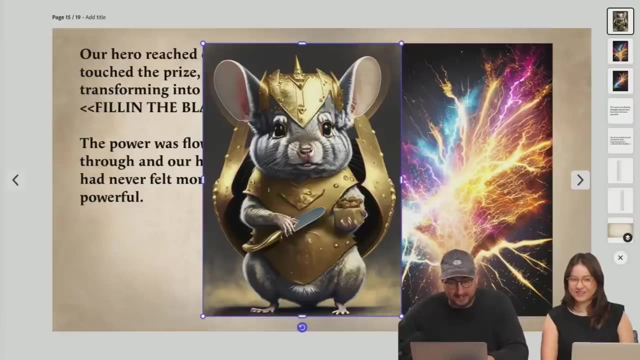 because what I want to do is align these perfectly And then I'm going to turn the top one into a screen And that way we have we can put our hero in the middle and then animate like it like coming out. So our new friends chinchilla, and somebody said in gold armor, hold on, look at his. 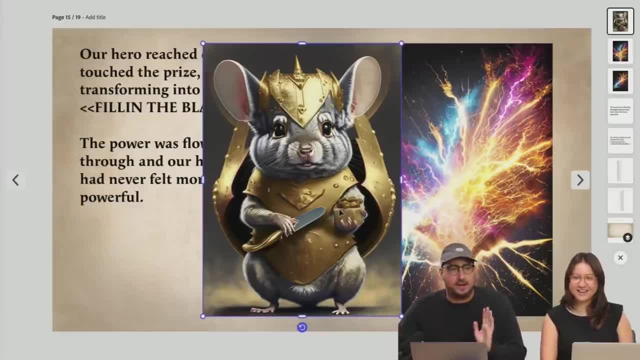 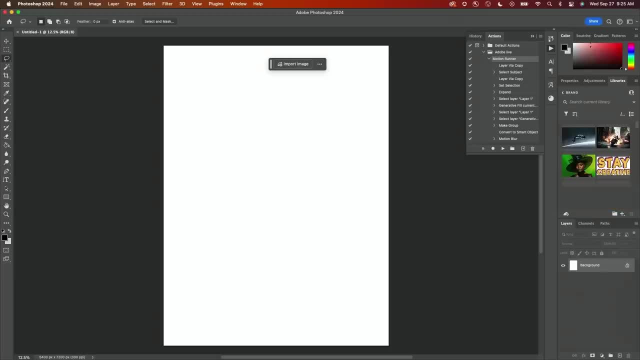 cheese knife And then he's got little charcuterie. Okay, So this guy is iconic, obviously. So I'm actually going to remove the background on this guy. Let's add to brand or library and I'll just add them to a library And you can see. now I am over in Photoshop and I'm going to find them right. 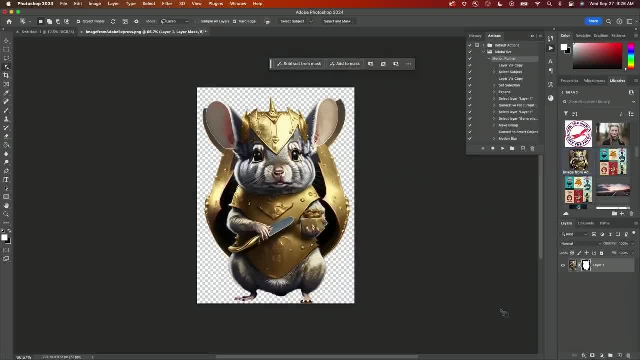 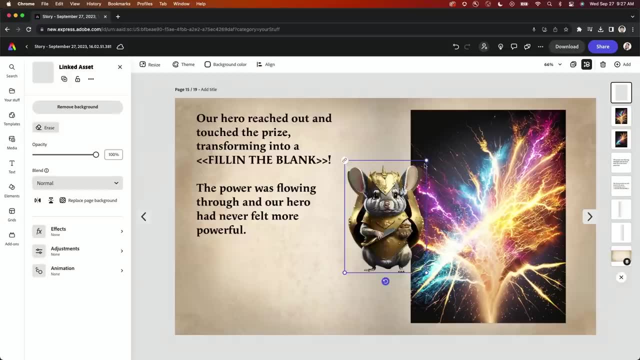 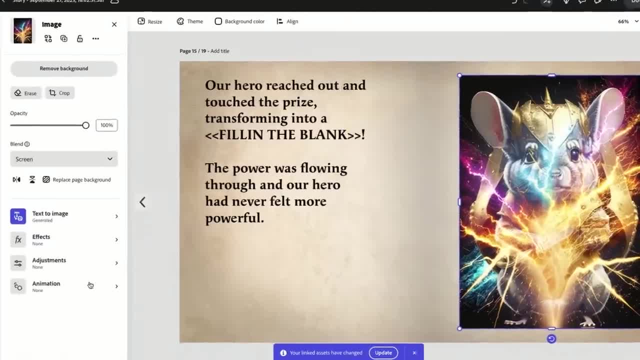 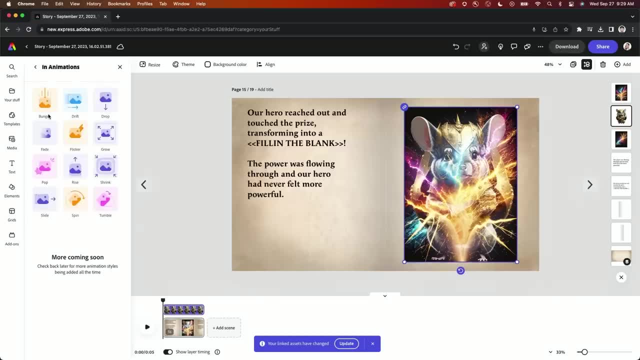 Kind of like explosion effect. I'm going to flicker, do an animation and we are going to go in. We are going to go flicker, Yeah. So we're going to go in and we are going to grow and let's do. 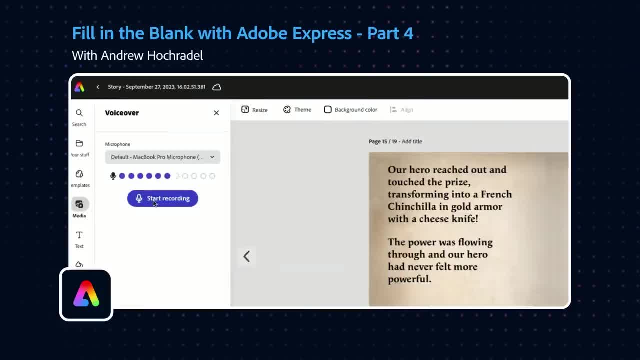 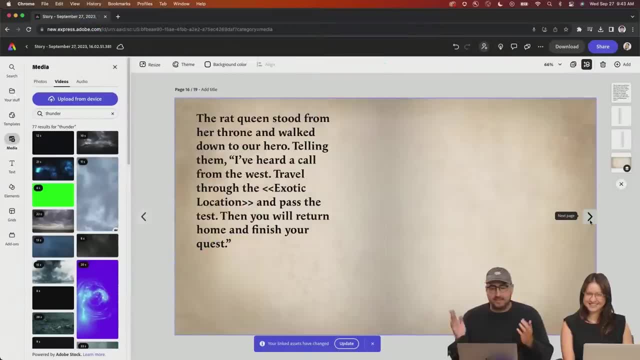 smooth. Now let's do our voiceover and our music. Our hero reached out and touched the prize, transforming into a French chinchilla in gold armor with a cheese knife. Guess what? The rat queen has something to say. What is this exotic location? 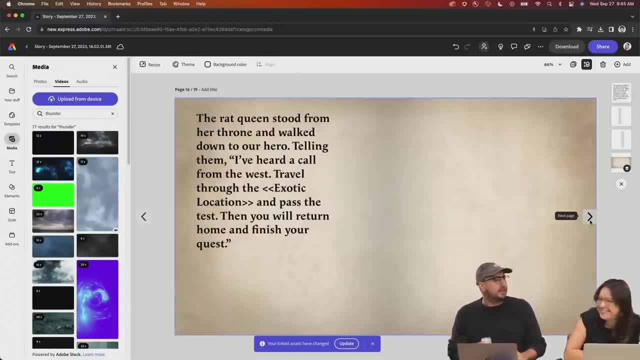 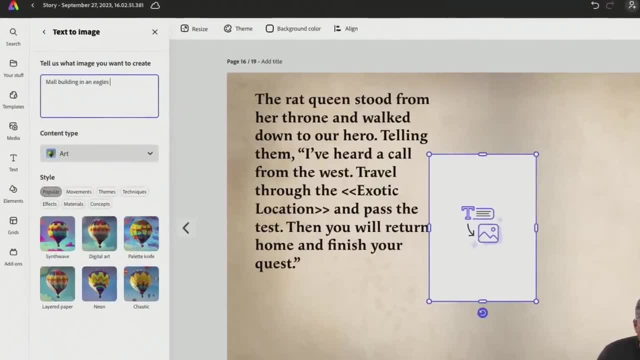 What does this location look like? Somebody's saying a sky mall. We could do sky mall in Eagle's nest. Okay, Photos, text, image. Here we go, A mall building in an Eagle's nest floating on clouds in the sky. It has to be full right, It has to be. 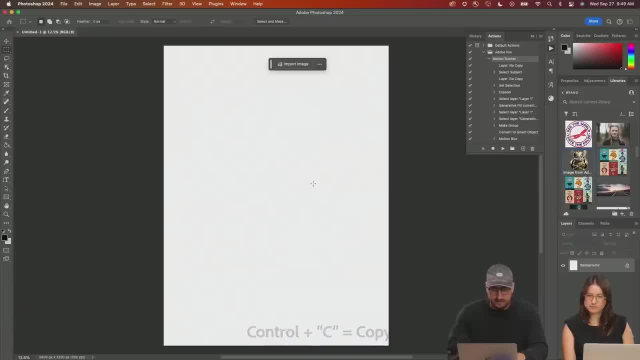 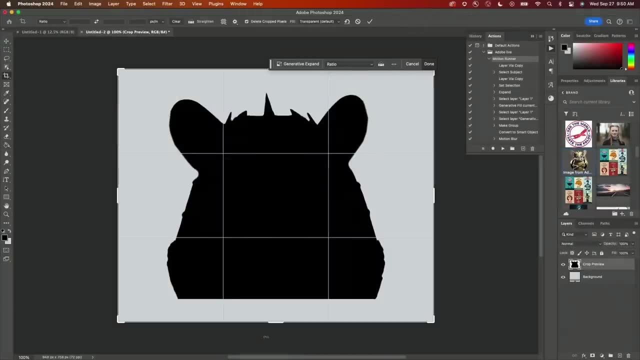 So we're going to have our hero here and I'm going to copy control C and then I'm just going to do it in Photoshop. I'm just going to fill this whole thing with black. So we're going to expand this out a little bit. We're just going to go to filter.